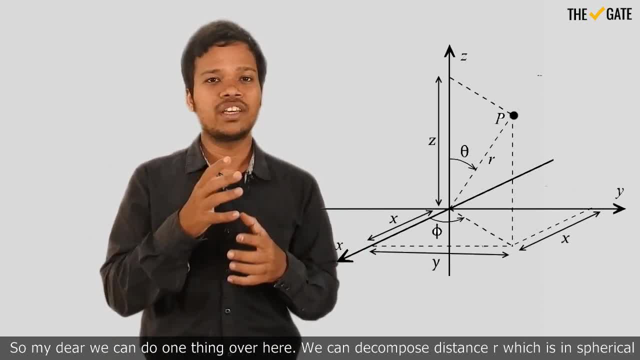 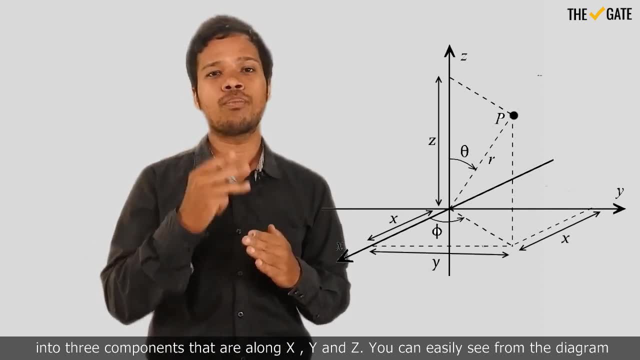 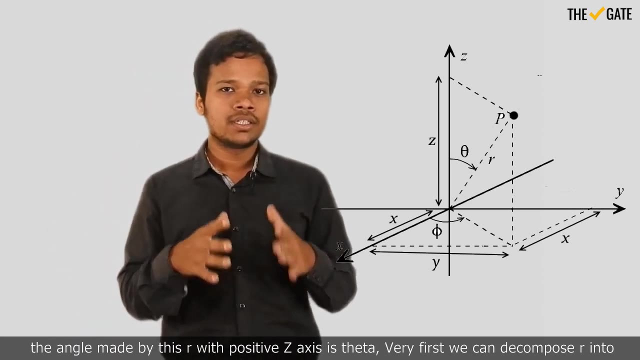 along Z axis. So, my dear, we can do one thing over here. We can decompose the distance R, which is in spherical, into three components that are along X, Y and Z. You can easily see from the diagram the angle made by this R with positive Z axis is equal. 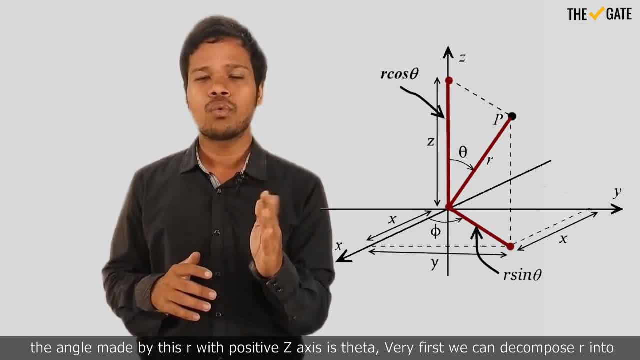 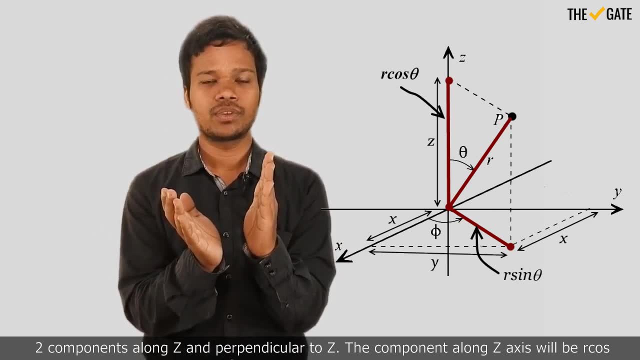 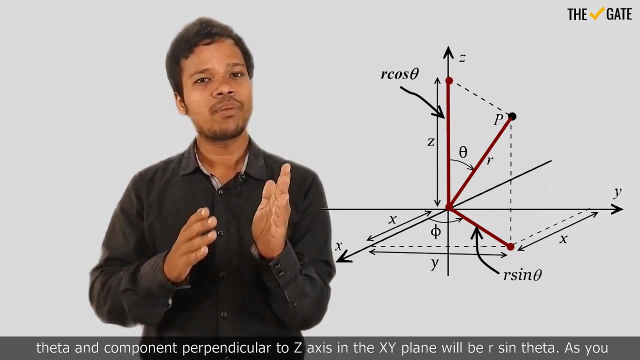 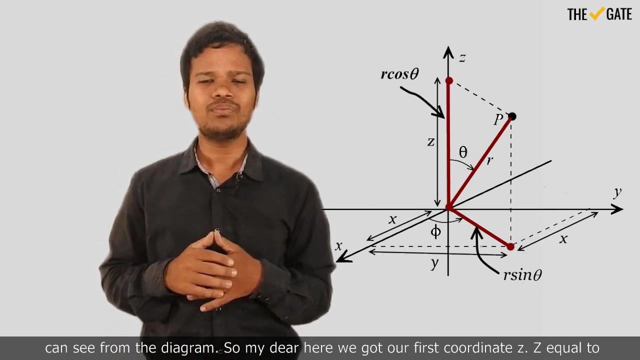 to theta. So in very first we can decompose this R into two components: along Z and perpendicular to Z. The component along Z axis will be R cos theta, and the component perpendicular to Z axis in the X Y plane will be R sine theta, as you can see from the diagram. 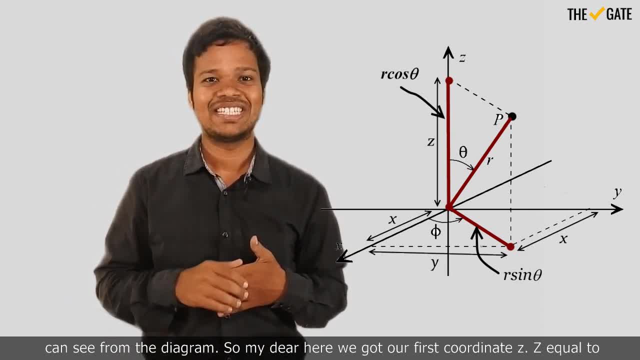 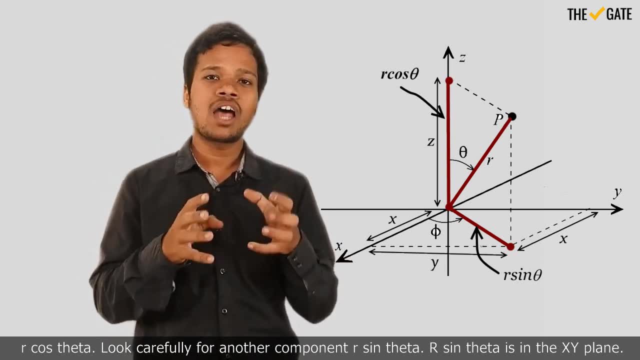 So, my dear, here we got our first coordinate Z Z equal to R sine theta. So now we have our first coordinate, Z Z equal to R sine theta. Look carefully for the other component, R sine theta. R sine theta is in the X Y plane. 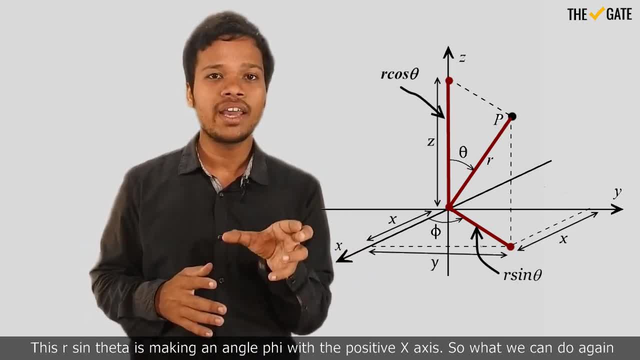 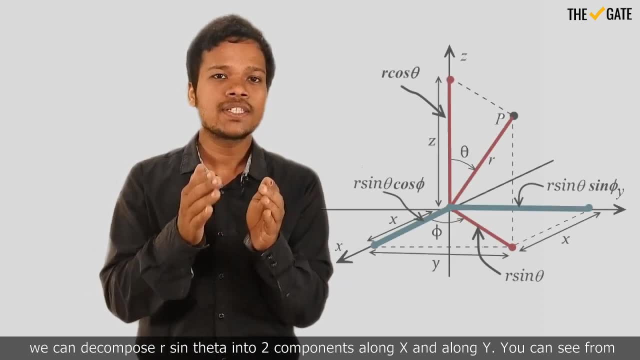 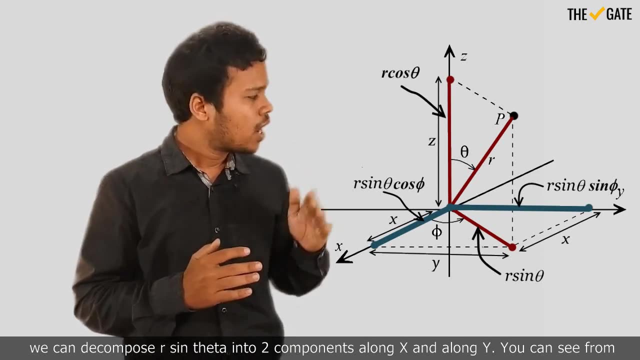 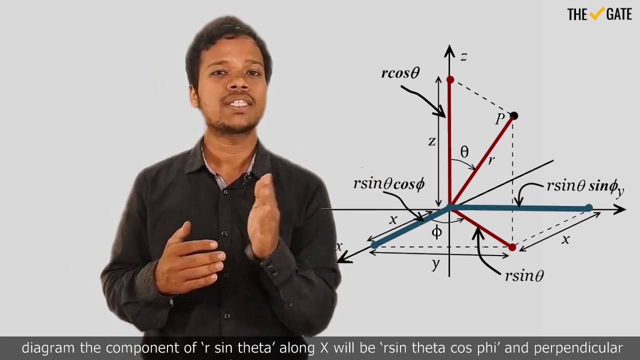 This R sine theta is making an angle Phi with the positive X axis. So what we can do again, we can decompose this R sine theta into two components, along X and along Y. You can see from the diagram: The component of R sine theta along X will be R sine theta, cos phi and perpendicular. 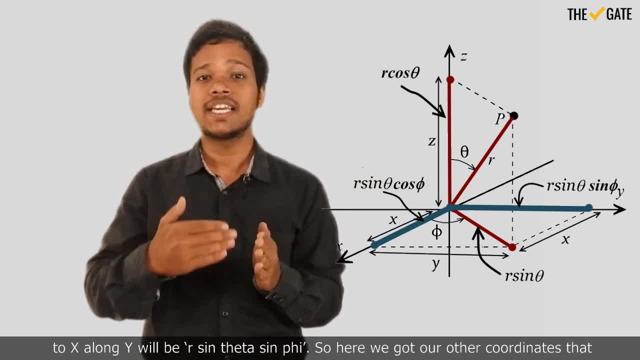 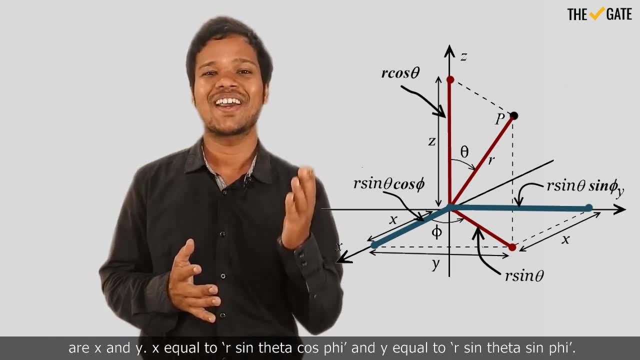 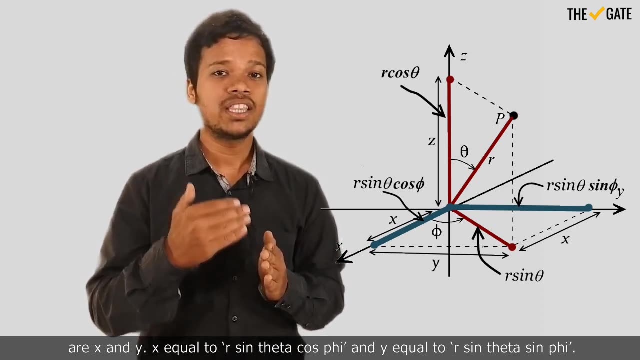 to X means along Y will be R sine theta sin phi. So here we got our other coordinates, that are X and Y, X equal to R sine theta cos phi and Y equal to R sine theta sin phi. So you know, this is very simple. 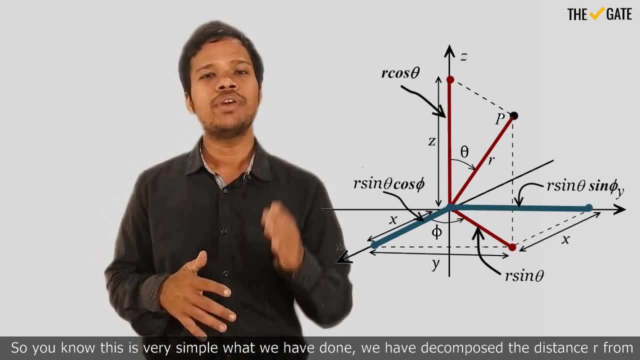 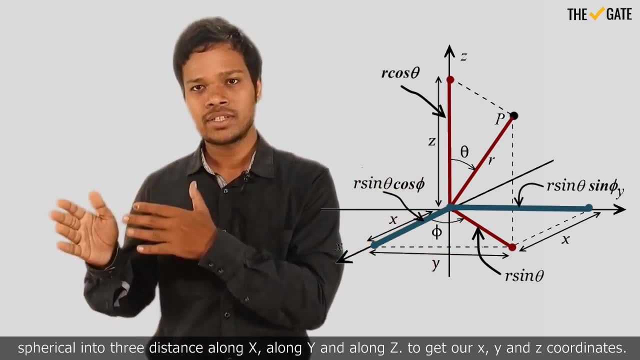 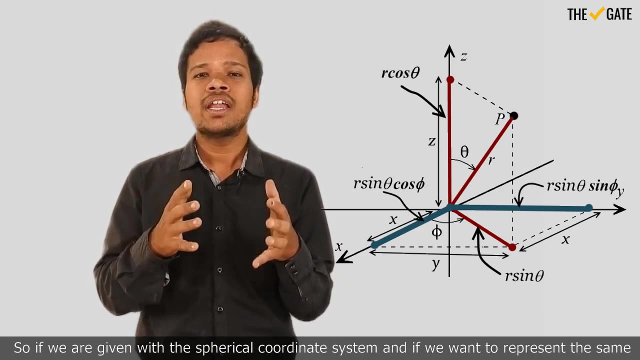 We have two coordinates. We have two coordinates. What we have done, we have decomposed the distance r from spherical into three distances, in along x, along y and along z, to get our x, y, z coordinates. So if we are given with the spherical coordinate system and if we want to represent the same point into cartesian, 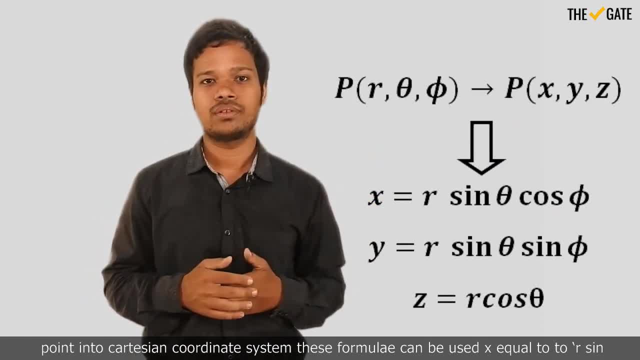 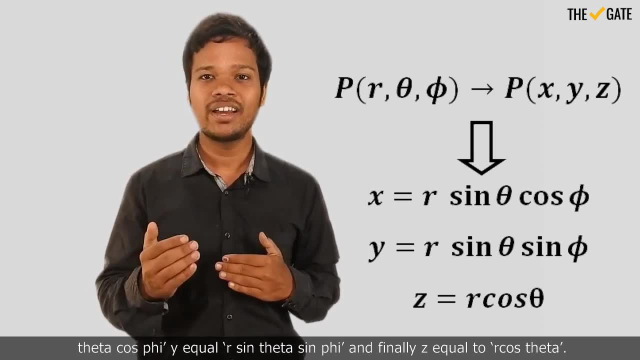 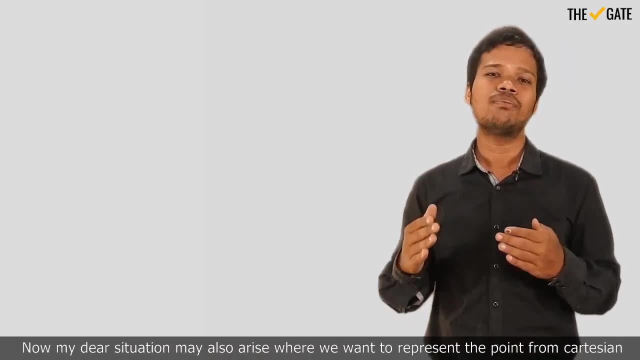 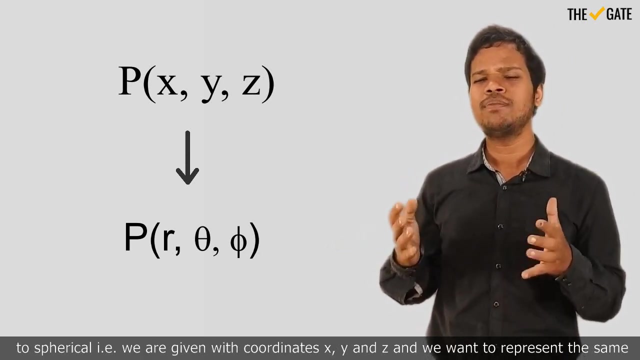 coordinate system. these formulae can be used: x equal to r sine theta cos phi, y equal to r sine theta sine phi and finally, z equal to r of cos theta. Now my dear situation may also arise where we want to represent the point from cartesian to spherical. That means we are given with coordinates. 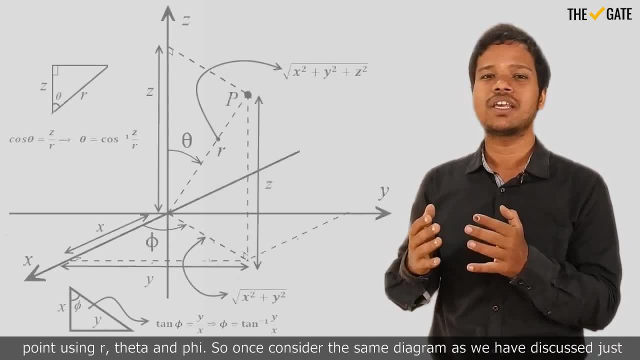 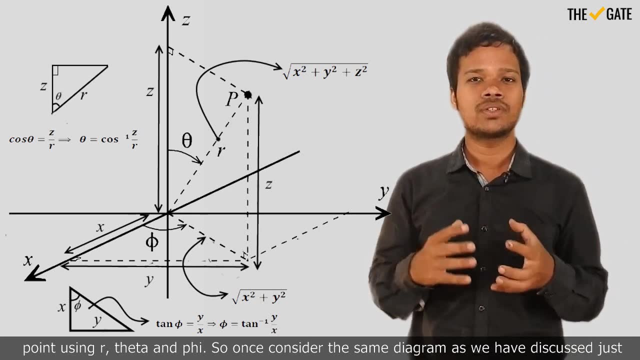 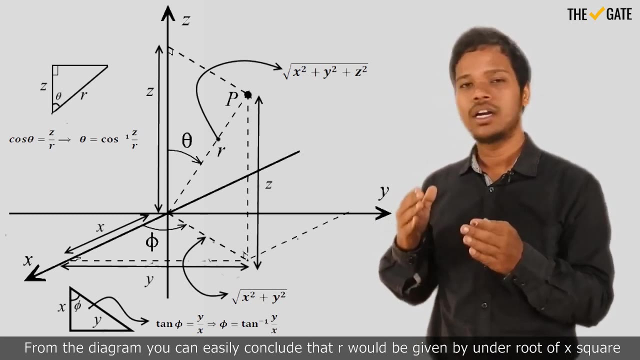 x, y and z, and we want to represent the same point Using r, theta and phi. So once again, consider the same diagram as we have discussed just now. From the diagram you can easily conclude that r would be given by under root of x. 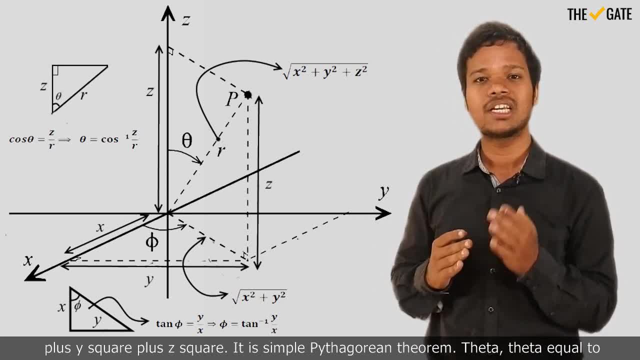 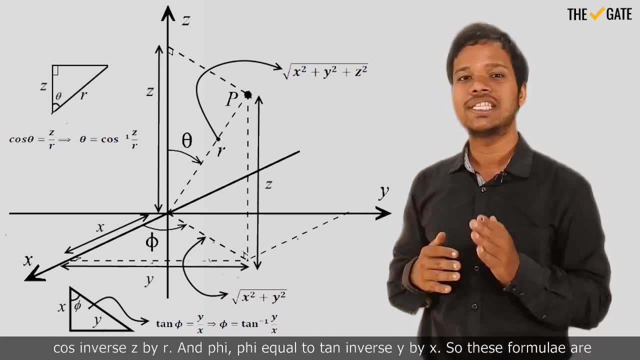 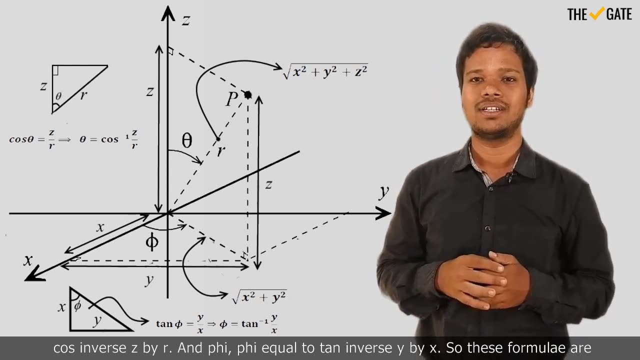 square plus y square plus z square. It is simple pythagorean theorem: Theta equal to cos inverse z by r, And phi equal to tan, y equal to phi inverse y by x. So these formulae are used when we want to represent any point from Cartesian. 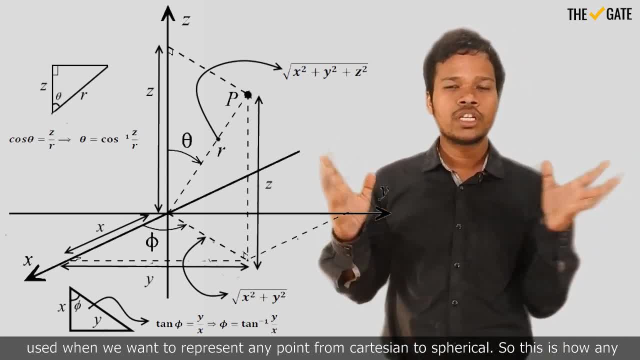 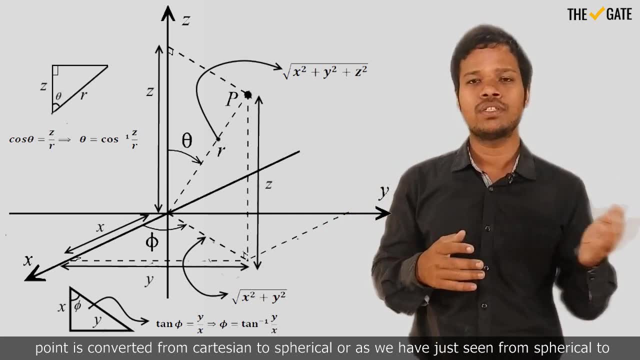 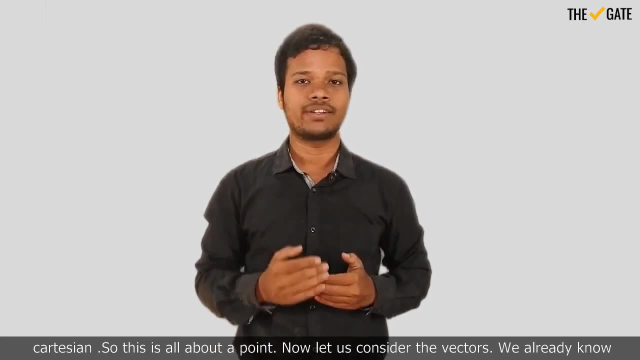 to spherical. So this is how any point is converted from Cartesian to spherical or, as we just seen, from spherical to Cartesian. So this is all about a point. Now let us consider the vectors. Now we already know that any vector in Cartesian coordinate system is: 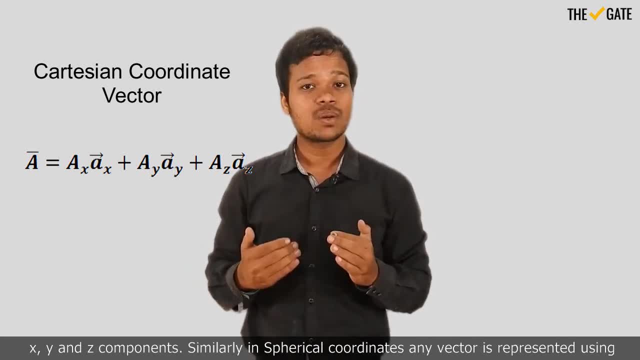 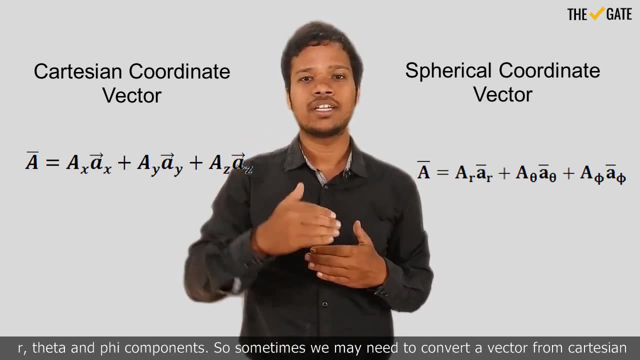 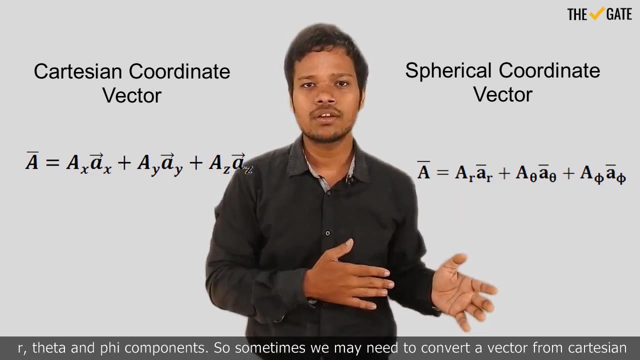 represented using three components, that are x, y and z component. Similarly, in spherical coordinates vector is represented using theta and phi components. So sometimes we may need to convert a vector from Cartesian to spherical or from spherical to Cartesian, In other words. 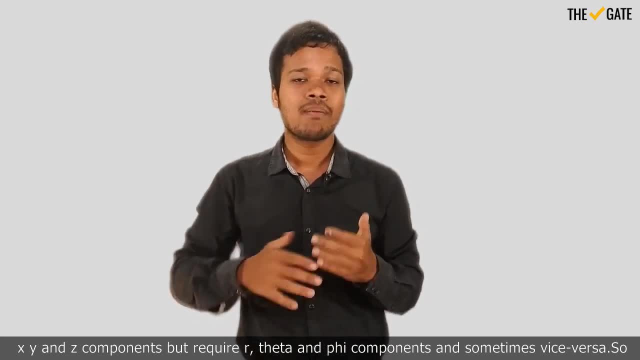 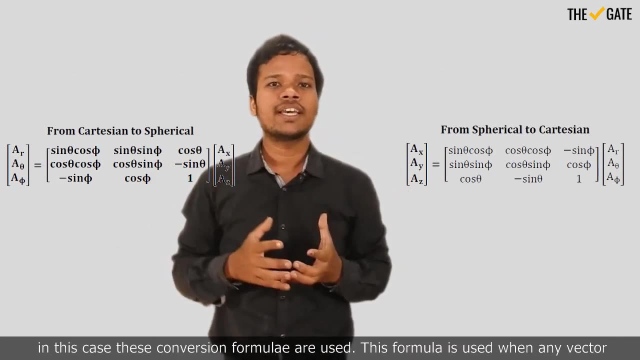 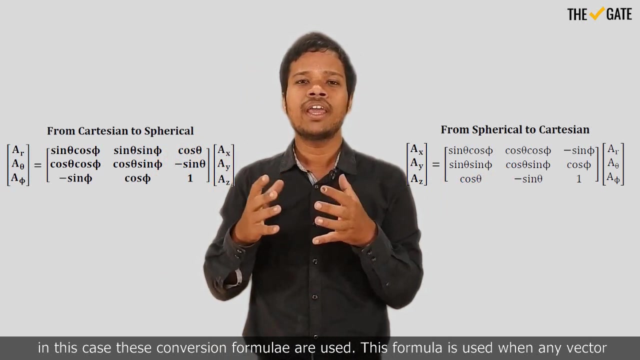 sometimes we are given with x, y and z components but require r, theta and phi components, and sometimes vice versa. So in this case these conversion formulae are used. This formulae is used when any vector from Cartesian is represented using spherical coordinate system. That means we: 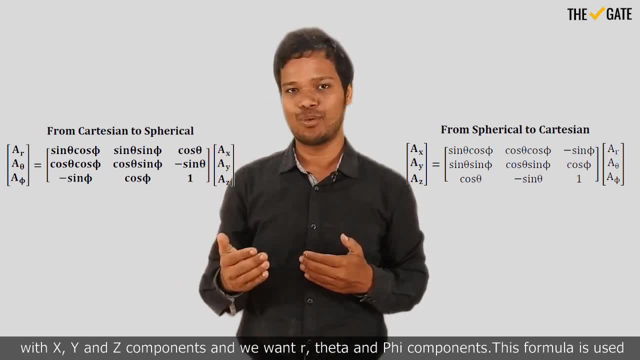 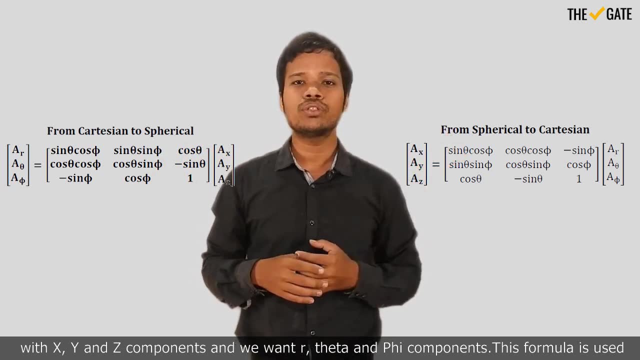 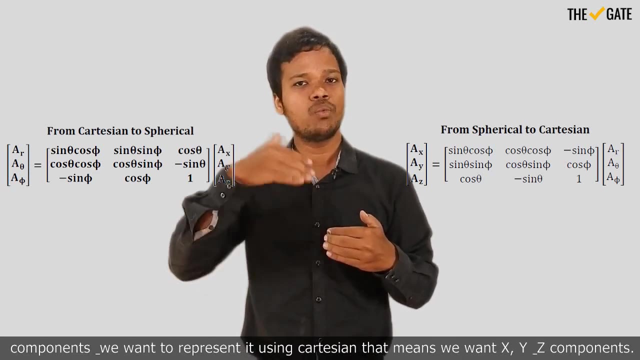 are given with x, y and z components and we want r, theta and phi components. So in this case we have r, theta and phi components. This formulae is used when we are given with spherical vector. That means we are given with r, theta and phi components and we want 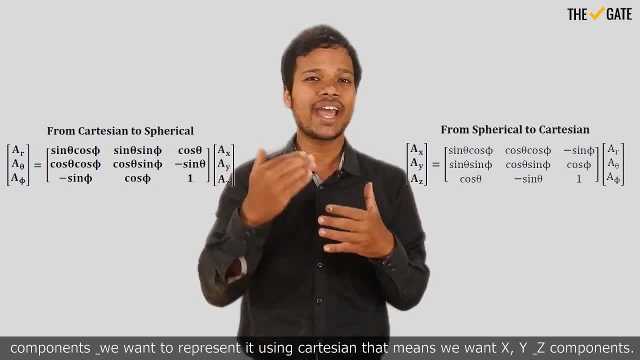 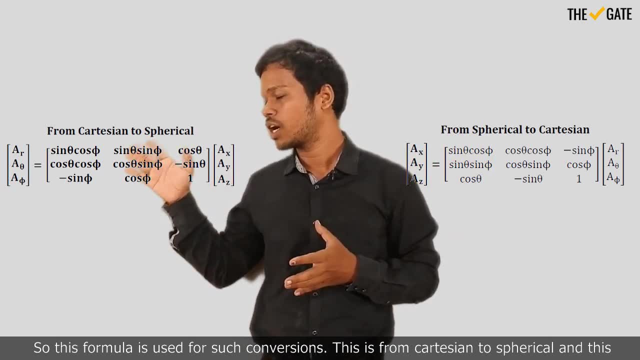 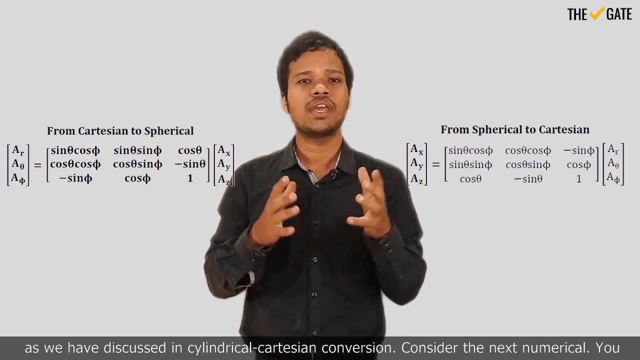 to represent it using Cartesian. That means we want x, y and z components. So this formulae used for such convergence. This is from Cartesian to spherical and this is from spherical to Cartesian. You know, the method of application is exactly the same as we have discussed. So 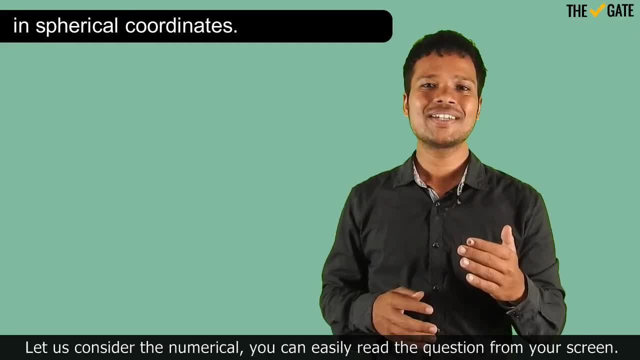 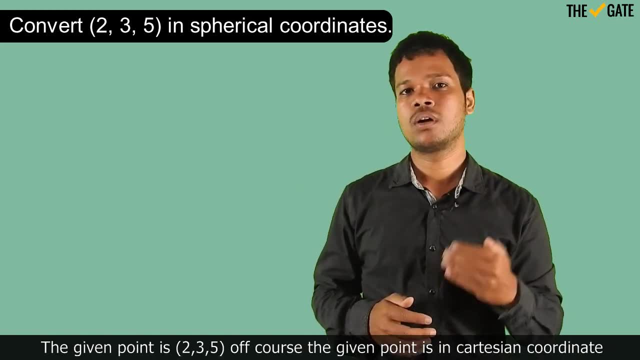 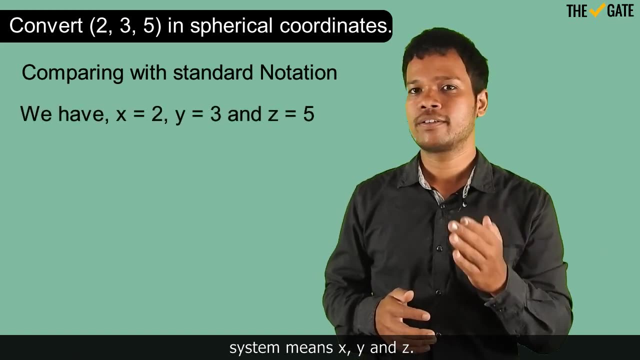 in cylindrical Cartesian conversion. Let us consider the numerical. You can easily read the question from your screen. The given point is 2,, 3, 5.. Of course, the given point is in Cartesian coordinate system. It is x, y and z. We are given with x equal to 2, y equal to 3. 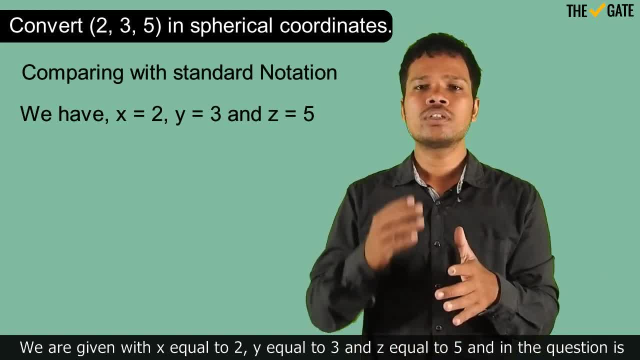 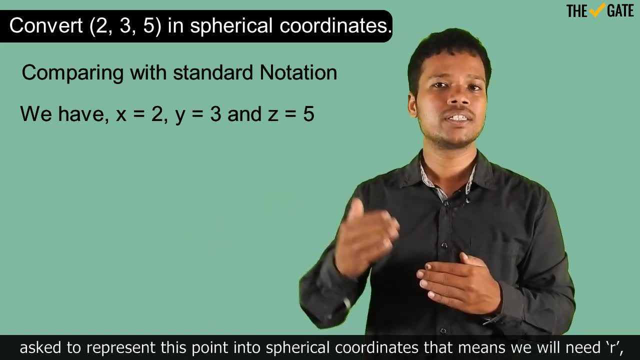 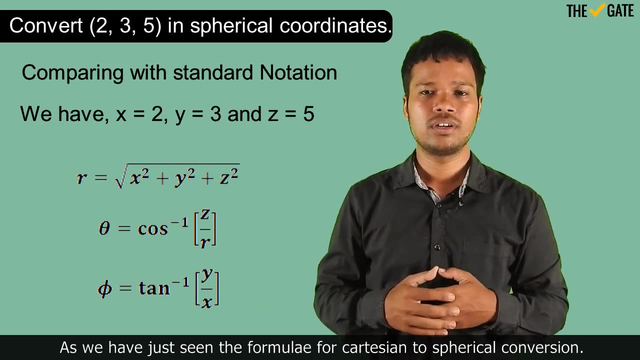 and z equal to 5.. And in the question it is asked to represent this point into spherical coordinates. That means we will need r, theta and phi. As we have just seen, the formulae for Cartesian to spherical conversion, r, is given by under root of x square plus y square plus z square. 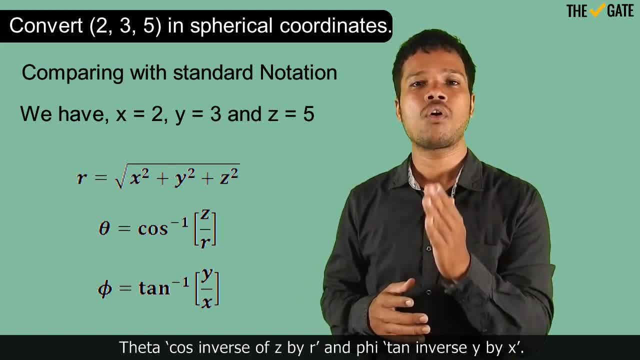 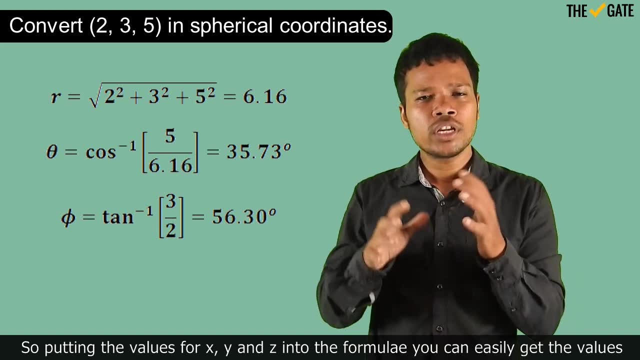 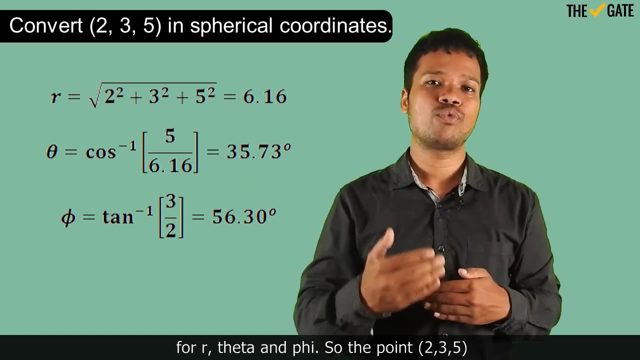 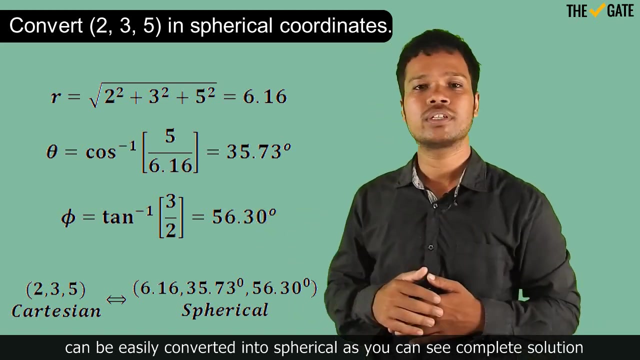 theta cos inverse of z by r and phi tan inverse y by x. So putting the values for x, y and z into the formulae You can easily get the values for r, theta and phi. So the point 2, 3, 5 can be easily converted. 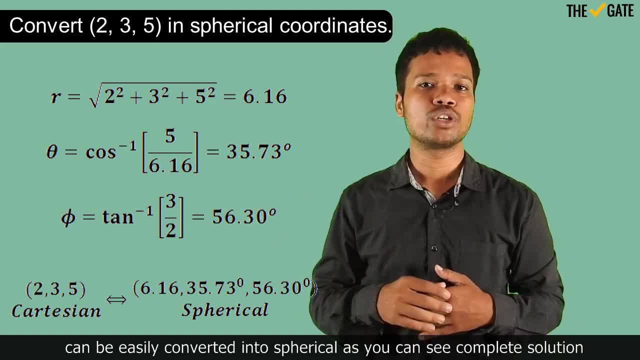 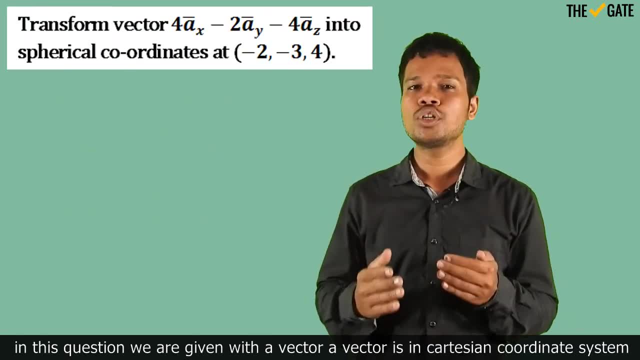 into spherical, As you can see complete solution on the screen. Let us take next numerical. You can read the question from your screen. In this question we are given with a vector. The vector is in Cartesian coordinate system. The given vector, as you can read. 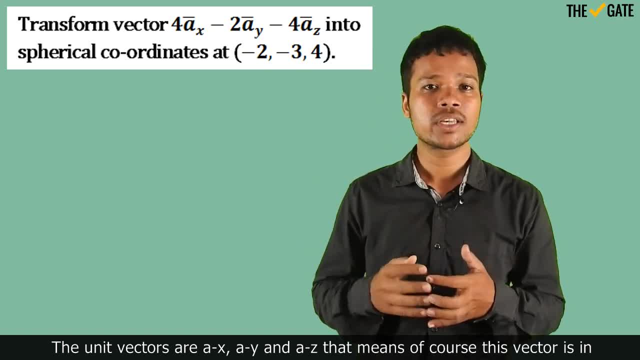 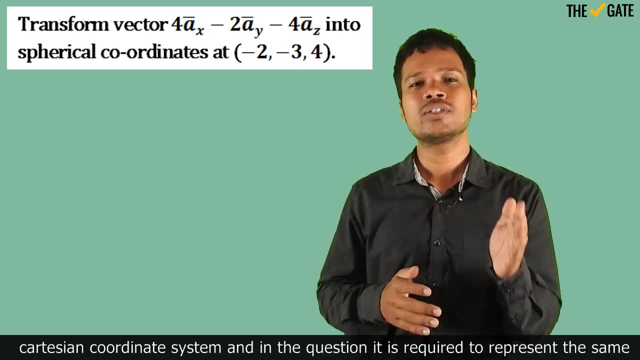 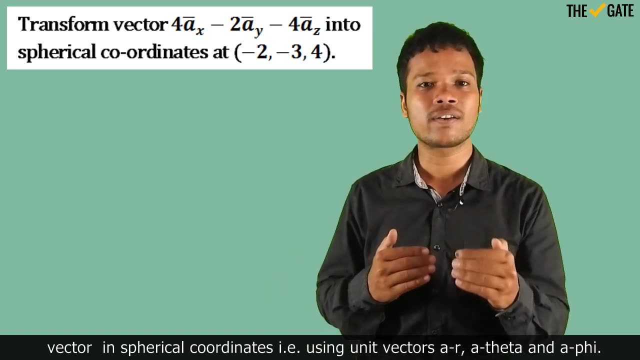 4, a z. The unit vectors are a, x, a, y and a z. That means of course this vector is in Cartesian coordinate system And in the question it is required to represent this same vector in spherical coordinates. That means using unit vectors a, r, a, theta and. 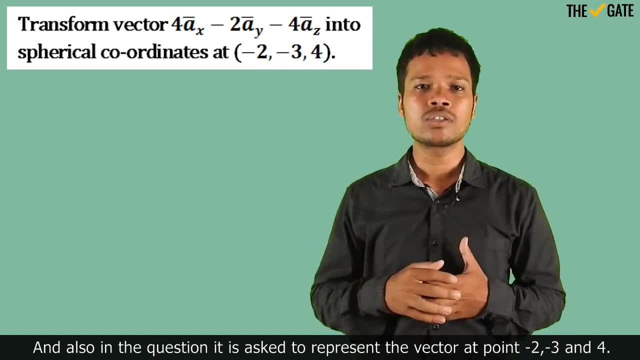 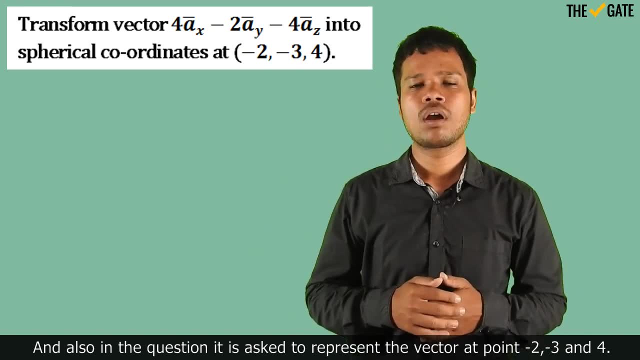 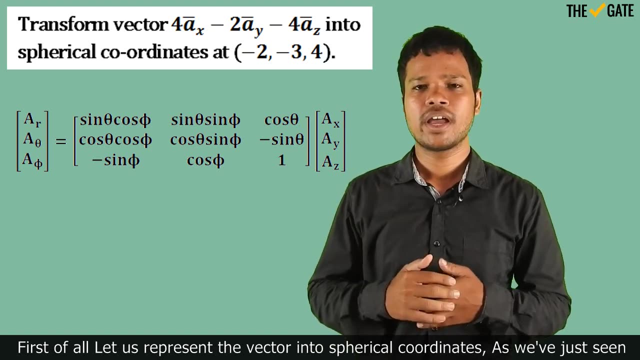 a phi And also in the question it is asked to represent the vector at point minus 2,, minus 3 and 4.. We will think about the point later. First of all, let us represent the vector into spherical coordinates, As we have just seen how to convert any vector from Cartesian to spherical or. 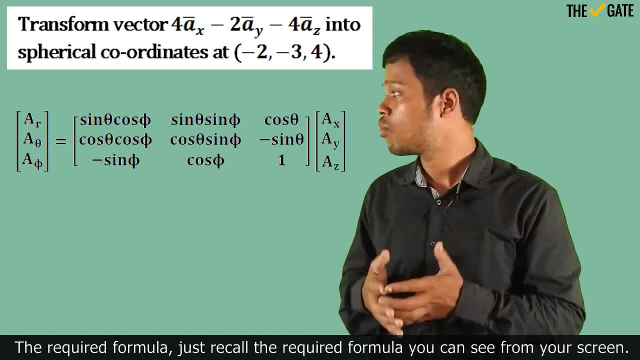 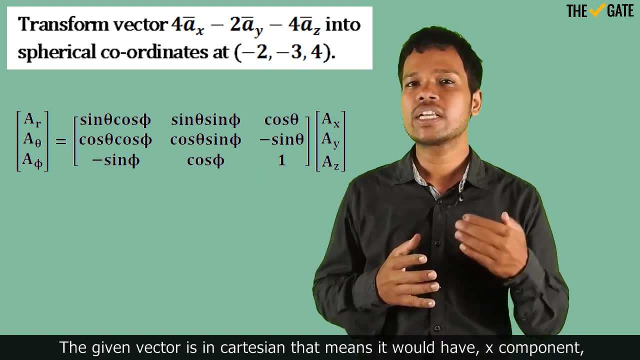 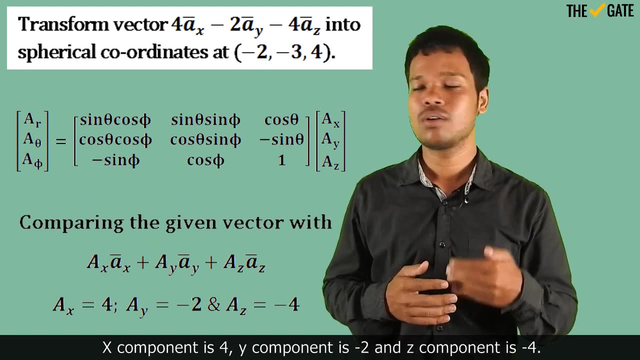 from spherical to Cartesian. The required formula. Just recall the required formula. you can see from your screen. The given vector is in Cartesian. That means it would have x component, y component and z component. X component is 4.. Y component is minus 2 and z component is minus 4.. So putting these x, y and z components 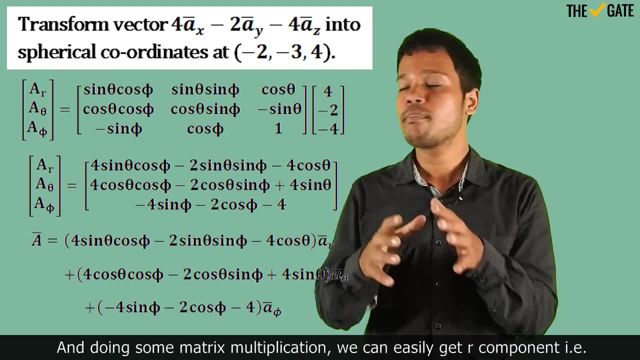 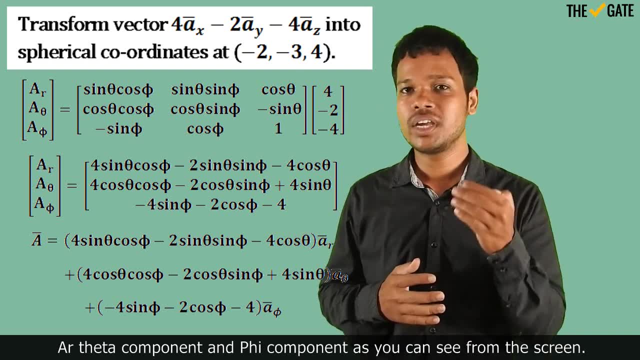 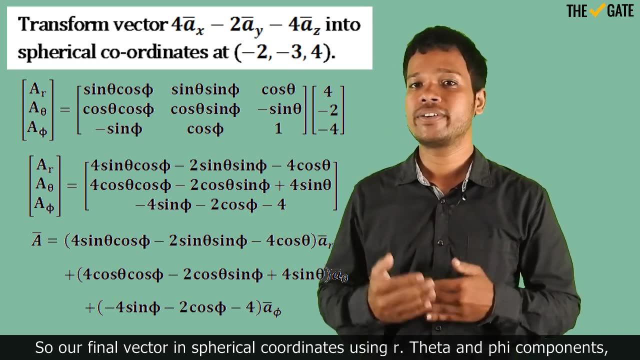 into your matrix formula and doing some matrix multiplication, we can easily get r component- that is, capital- AR, theta component and phi component, as you can see from the screen. So our final vector in spherical coordinates using r, theta and phi components. Let us see how to form this w back. 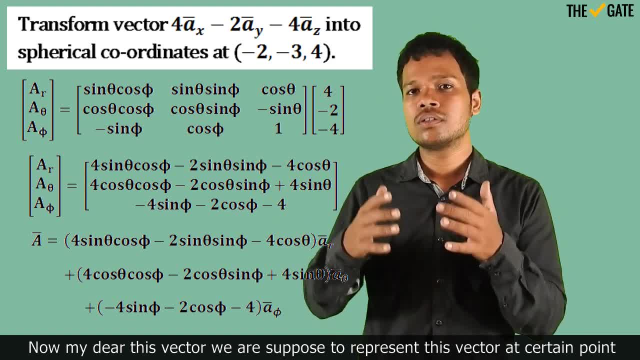 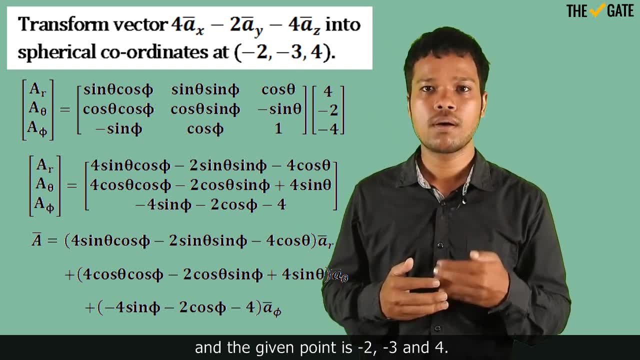 Let us write down type Corticoid for one of these vectors. So this vector is a 4- payroll vector. It will be represented by the different numbers. For example I have leaf drop. Other common sense for this is that these have each other � likeова minus 2, minus 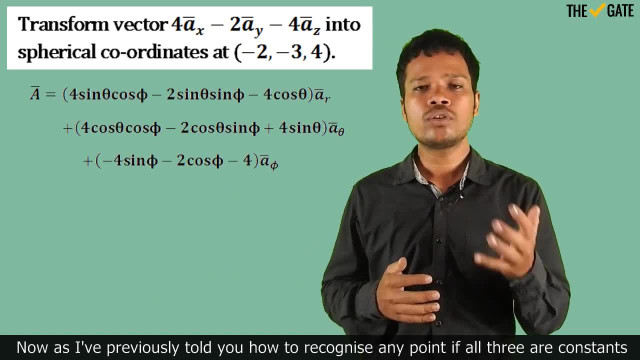 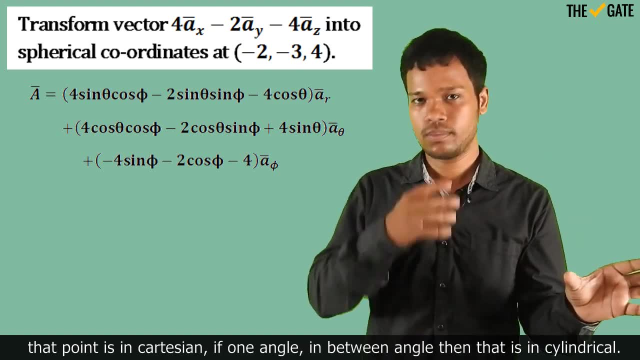 2 and 3.. Part謝, you can also use a number letter. If you have such numbers like that, you can read of them or marked as: Similarly: we consider this two and see if that means these match. ining values are: ahm. 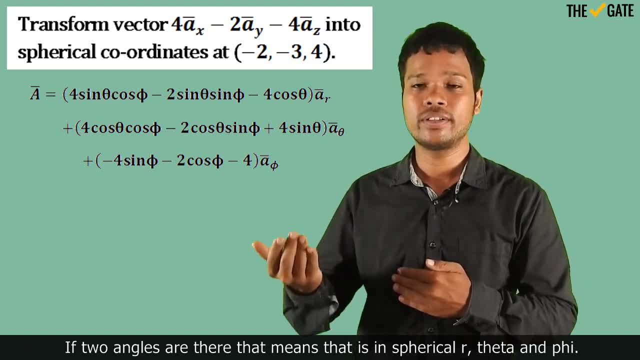 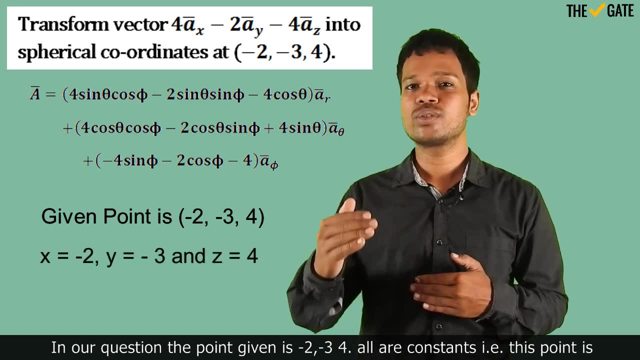 It applies both if all three things are constants. we write down thick: Now we should understand that this vector represents If two angles are there. that means that is in spherical r, theta and phi. In our question the point given is minus 2, minus 3, 4. all are constants. that means this point is in cartesian. 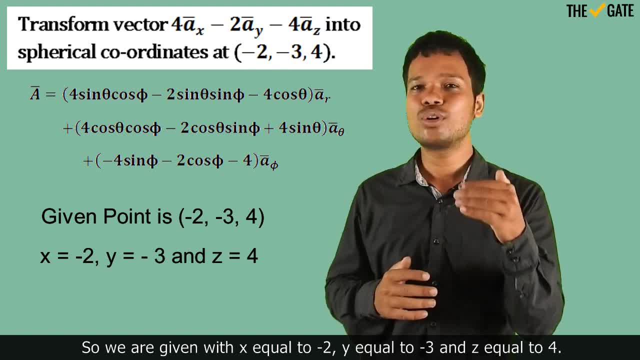 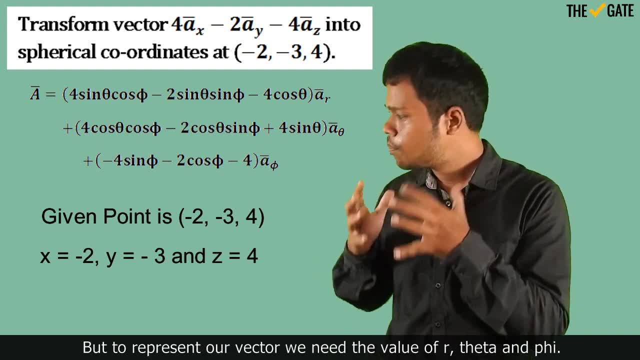 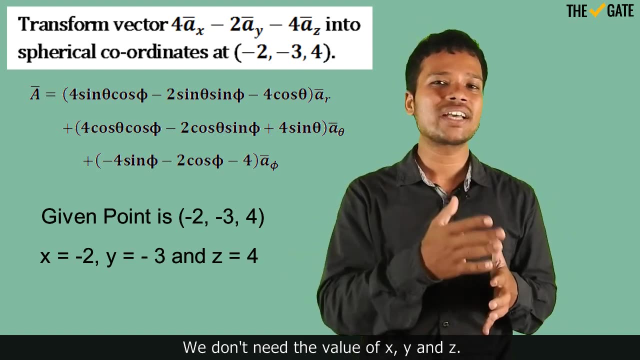 coordinate system. So we are given with x equal to minus 2, y equal to minus 3 and z equal to 4.. But to represent our vector we need the value of r, theta and phi. We don't need the value of x, y and 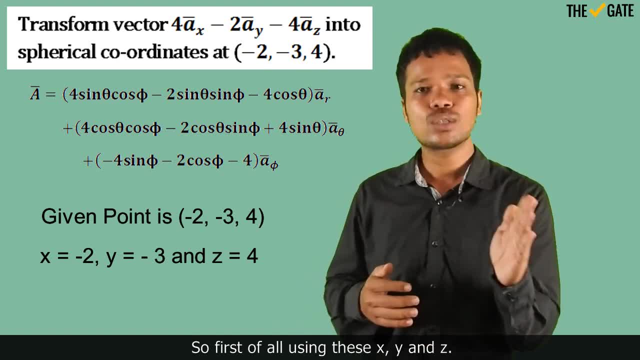 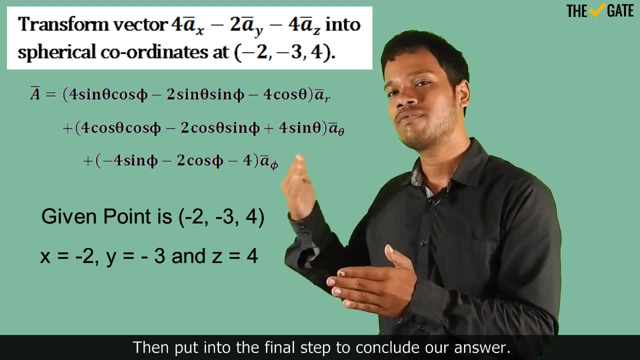 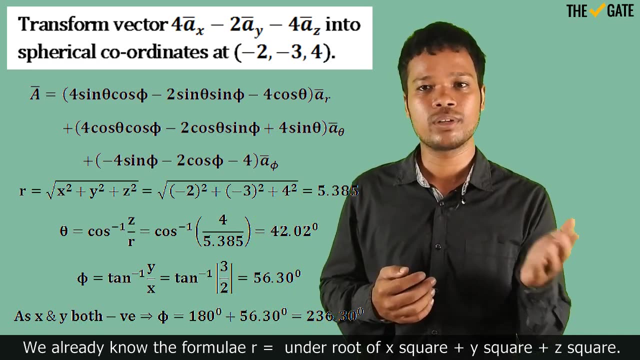 z. So first of all, using these x, y and z, let us first calculate r, theta and phi and then put into the final step, to conclude our answer. We already know the formulae r equal to under root of x square plus y square plus z square. 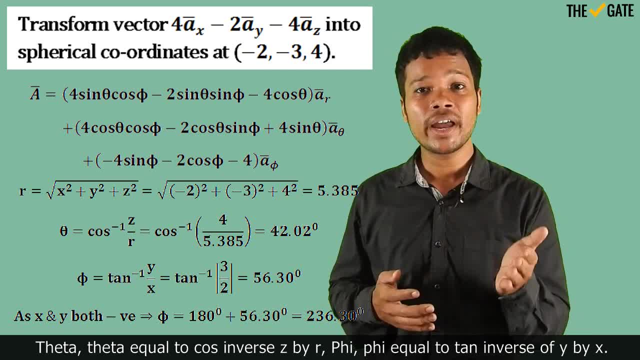 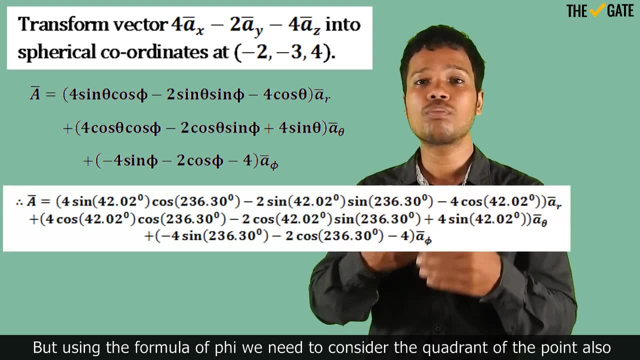 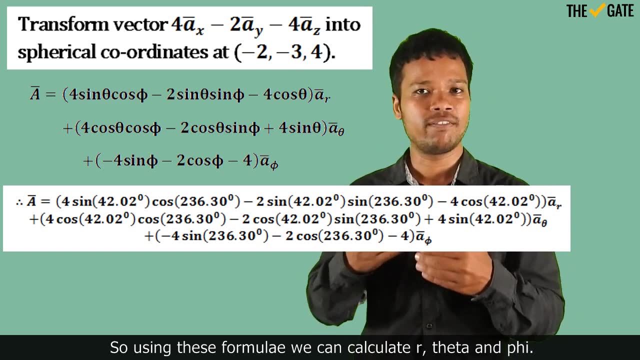 Theta equal to cos inverse z by r phi. phi equal to tan inverse y by x. But using the formula for phi, we need to consider the quadrant of the point also, as we have previously seen. So using this formulae you can calculate r, theta and phi and after getting the values of r, theta and phi, we 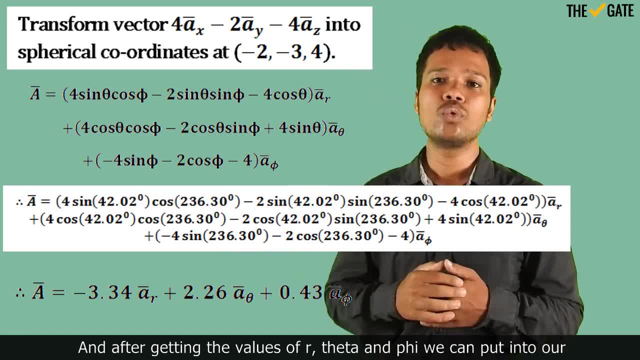 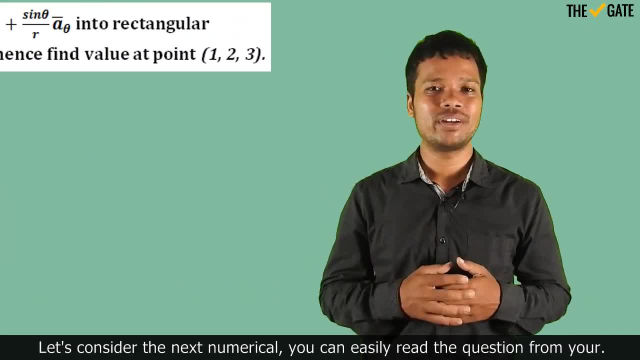 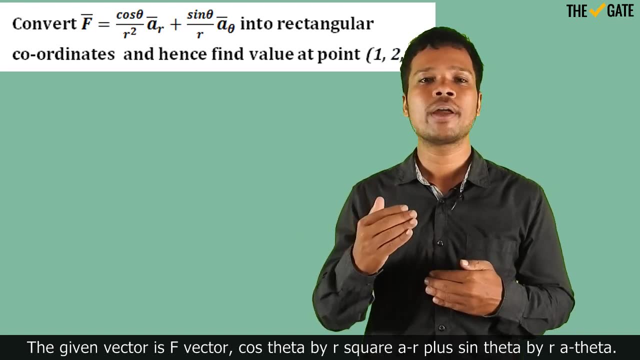 can put into our final step. to conclude the answer, as you can see from your screen, Let us consider the next numerical. You can easily read the question from its screen. The given vector is f vector cos theta by r square ar plus sine theta by r a theta. 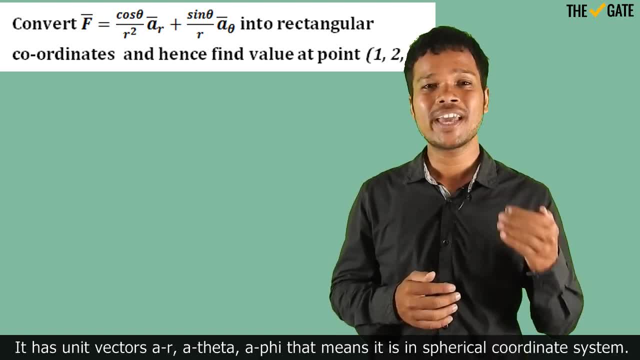 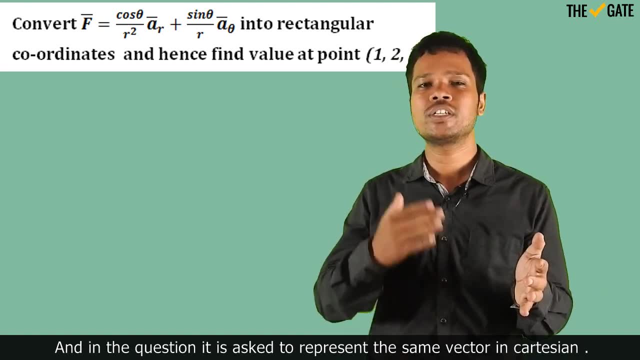 The given vector is in spherical coordinate system. It has unit vectors a, r, a, theta. that means it is in spherical coordinate system And in the question it is asked to represent the same vector into cartesian coordinates. that means in terms of ax, ay and az. 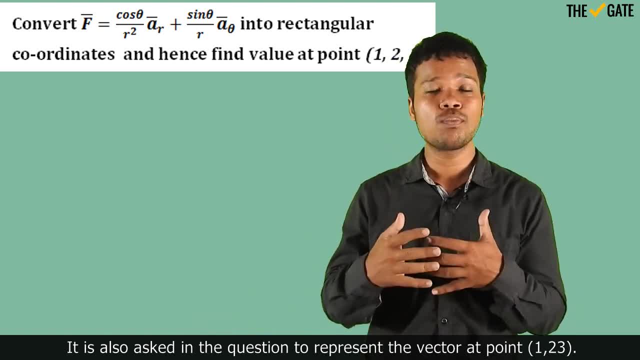 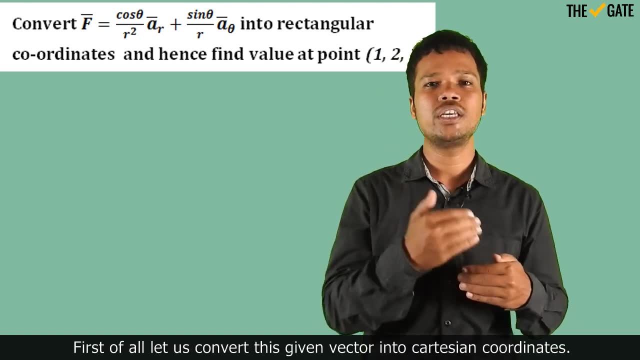 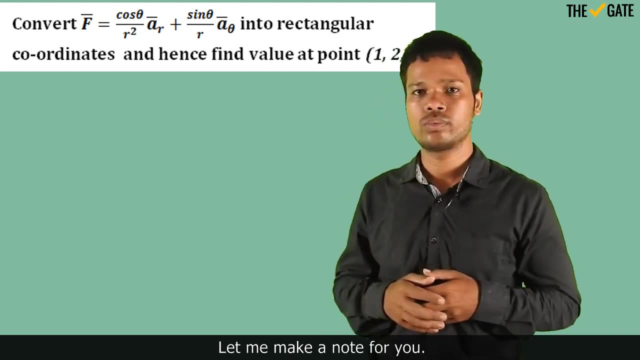 It is also asked in the question to represent the vector at point 1, 2 and 3.. We will see about the point later. First of all, let us convert this given vector into cartesian coordinates. But before also that, let me make you one note for you: In this vector, the r component, theta. 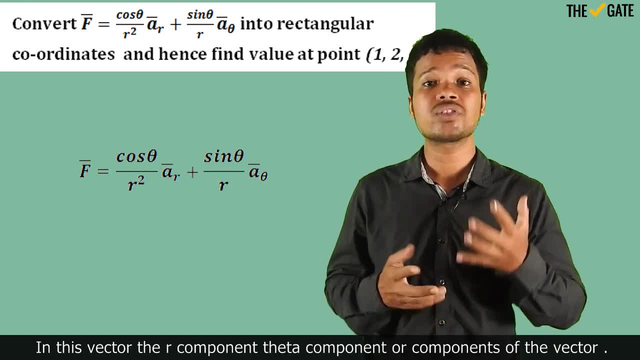 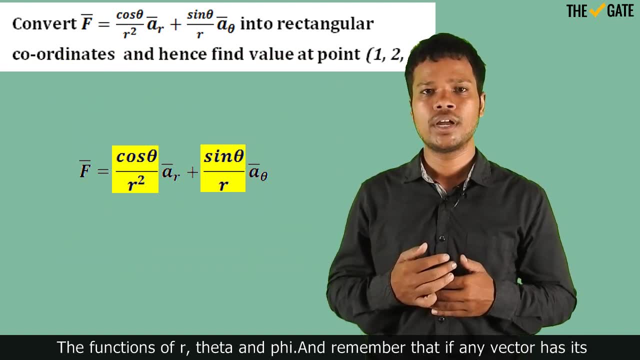 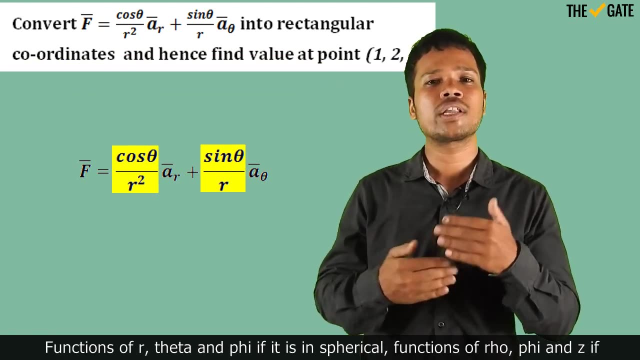 component or components of the vector are not constants. The components are certain kind of functions, Functions of r, theta and phi. And remember that if any vector has its components as a functions, Functions of r, theta, phi, if it is in spherical, Functions of rho, phi and 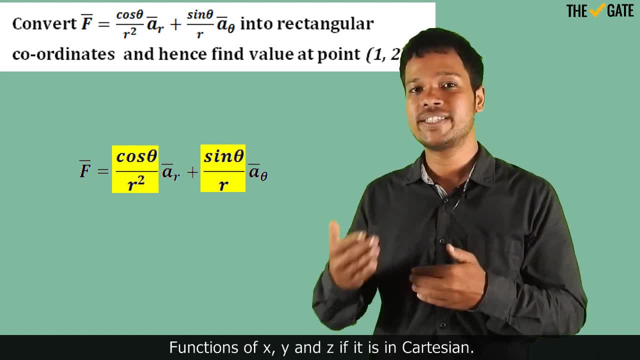 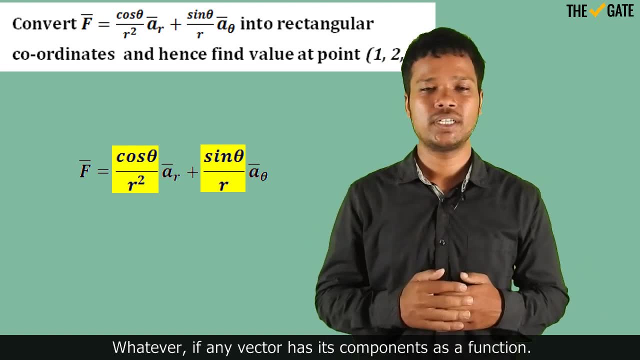 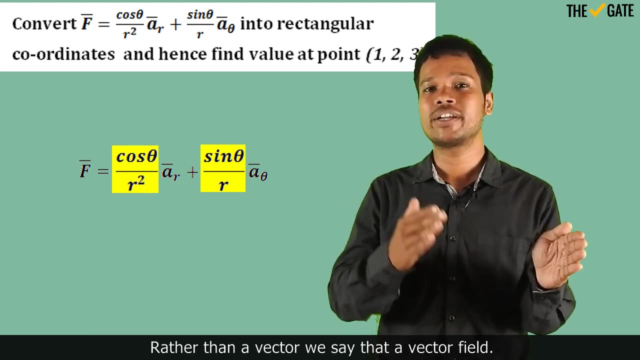 z if it is in cylindrical Functions of x, y and z if it is in cartesian. Whatever, If any vector has its components as a function, then such vector is called as a vector field rather than vector. So we say that a vector field. So actually we are given with vector field in this question. 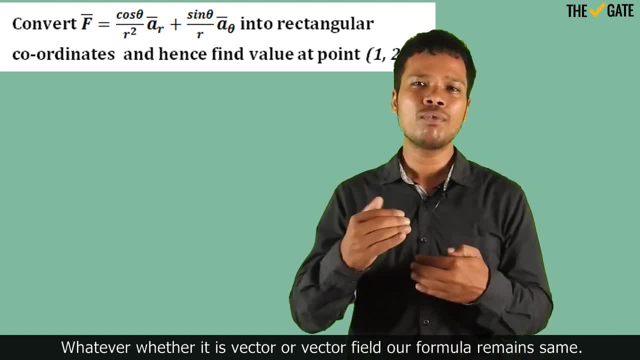 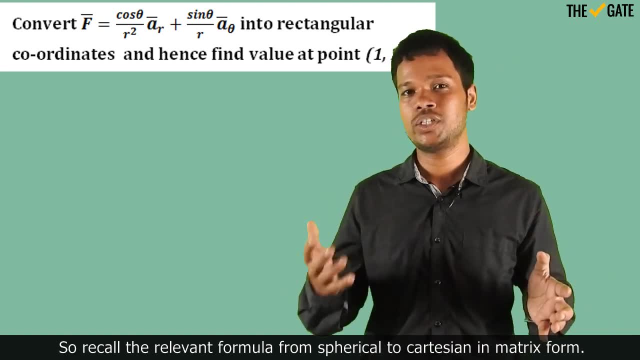 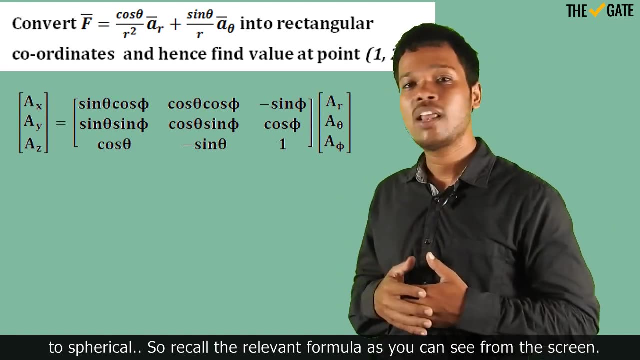 Whatever, whether it is a vector or vector field, our formula remains same. So recall the relevant formula for conversion from spherical to cartesian in matrix form. We have seen both the formulae from cartesian to spherical and from spherical to cartesian, So recall the relevant formula. as you can see from your screen, 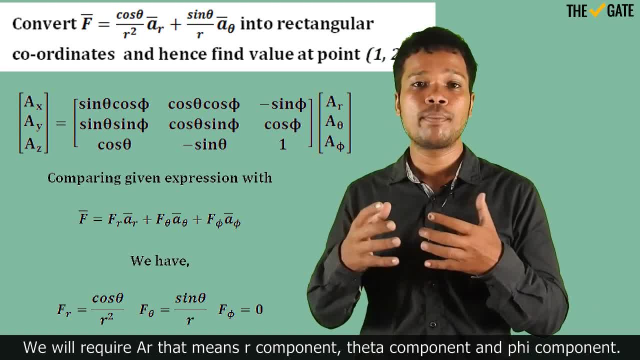 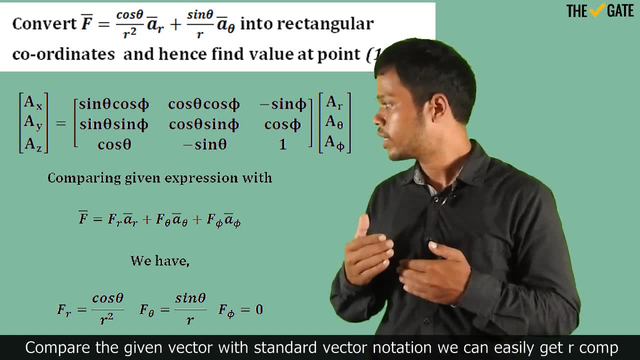 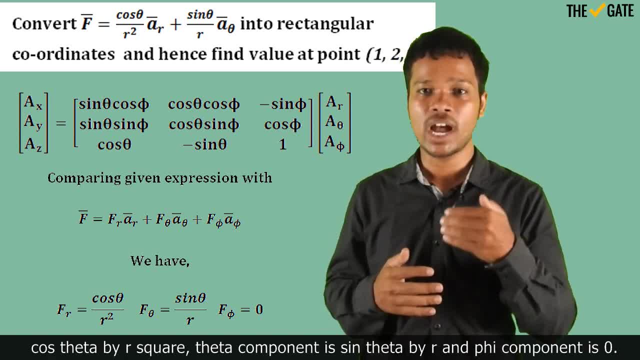 Rather thanressed to give us achauble from by kyive. depends upon ro capital. a r that means rho component, Theta component and phi component, The. compare the given vector with standard vector notation. we can easily get: r component is cost theta by r square theta. 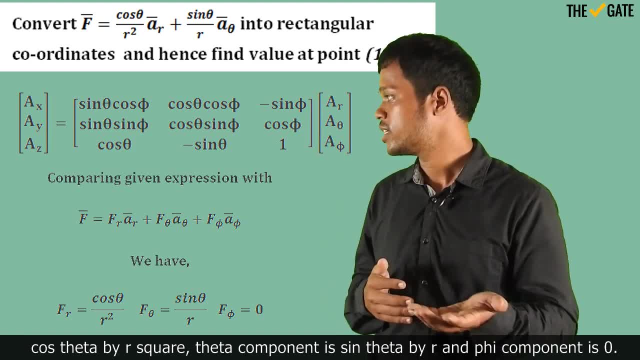 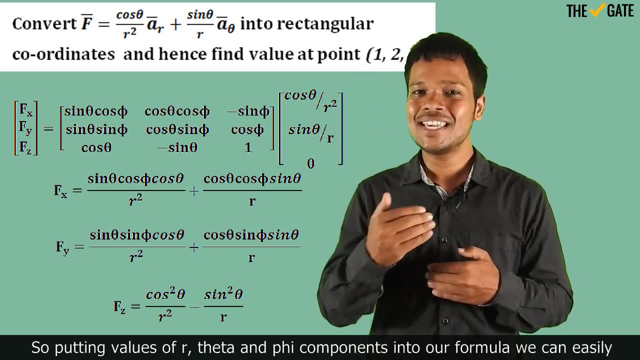 component is sine theta by r and phi component is zero. So putting values of r, theta and phi components into our formula, we can easily get values for x component, y component and phi component. asurarva, So each Expector zllie emand to equality. 그러니까 we have received the negative. 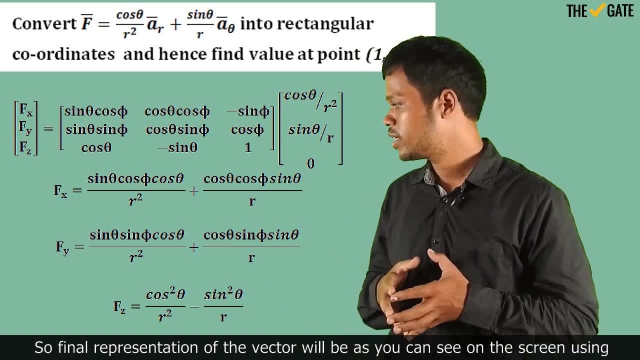 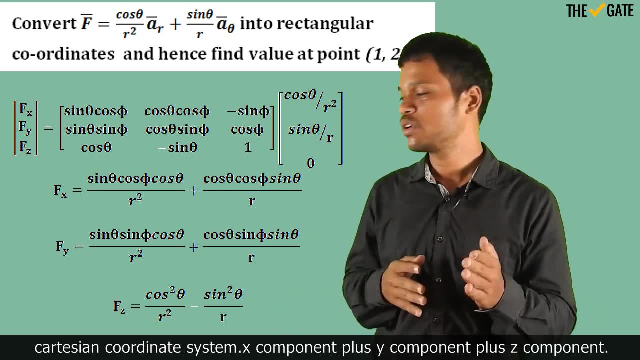 information that we have são in с範. Ronald insist in engineering that a function, an proof and z component. So final representation of the vector will be as you can see on the screen, using Cartesian coordinate system: x component plus y component plus z component. 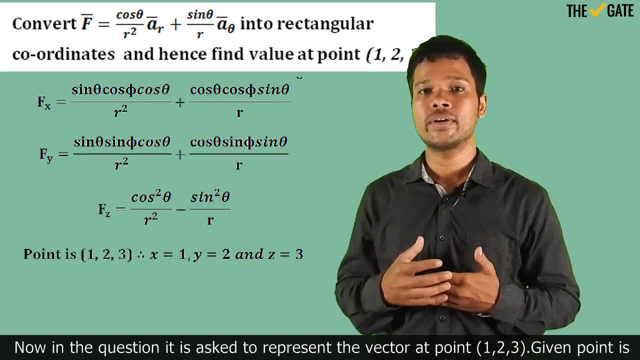 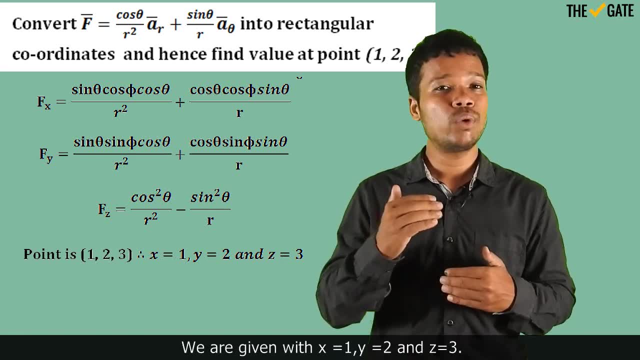 Now in the question it is asked to represent the vector at point 1,, 2, 3.. The given point is in Cartesian coordinate system. We are given with x equal to 1, y equal to 2 and z equal to 3.. 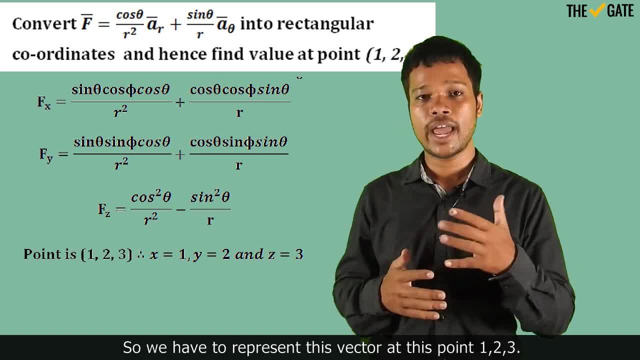 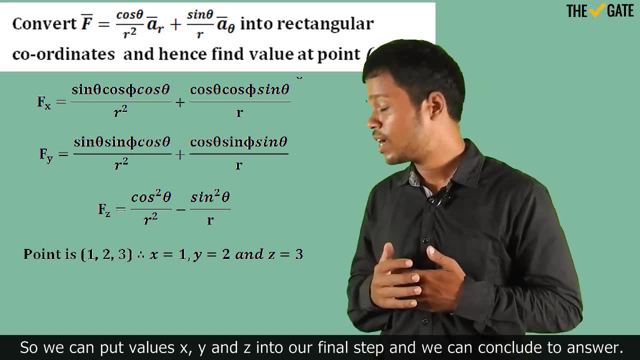 So we have to represent this vector at this point: 1,, 2,, 3.. So we can put values for x, y and z into our final step and we can conclude to our answer. But as you can see from your screen, 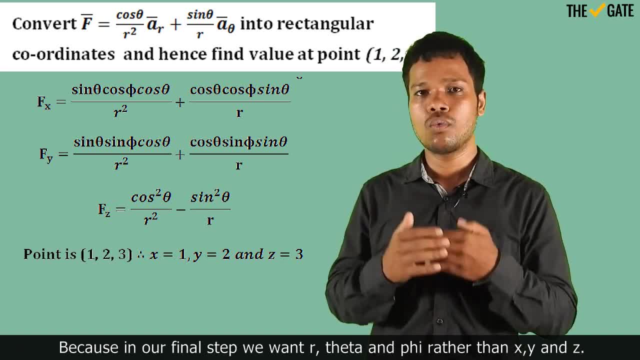 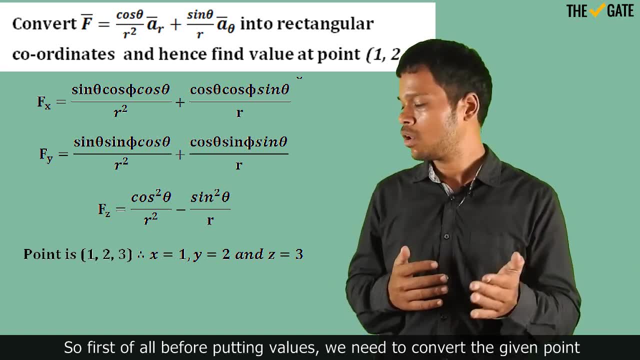 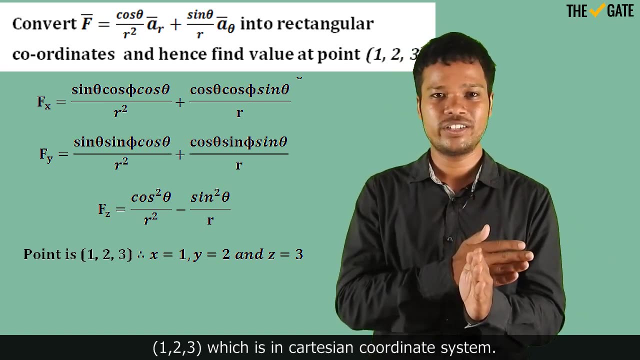 we can't Because in our final step we want r, theta and phi rather than x, y and z. So first of all, before putting the values, we need to convert the given point 1,, 2, 3, which is in Cartesian coordinate system. We have to convert this point into: 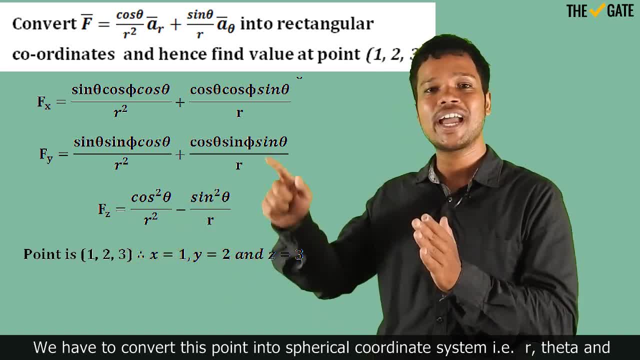 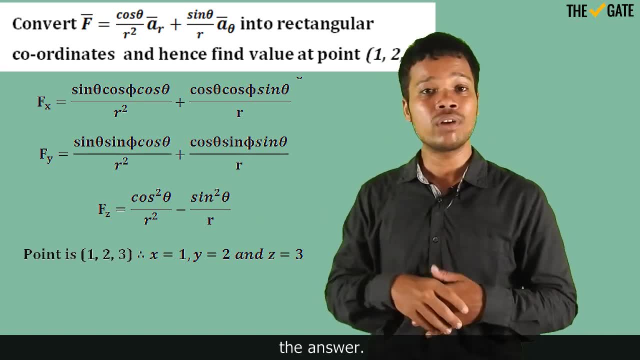 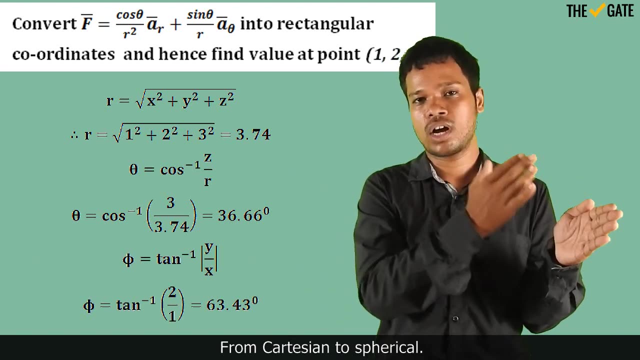 spherical coordinate system. That means r, theta and phi, So that we can put values of r, theta and phi into our final step and we can conclude to our answer. So we already know the formula from point conversion from Cartesian to spherical r equal to under root of x square plus y square.